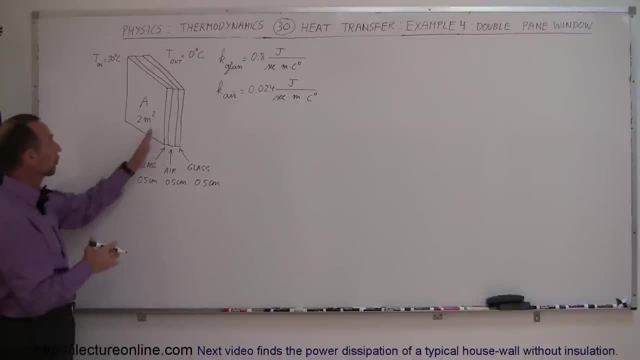 oversimplification. we're going to assume that those are indeed the temperatures of the inside piece of the glass and the outside piece of the glass, And of course in real life that's not the case. but just so for comparison to what we did before, The equation we normally use is dq- dt. 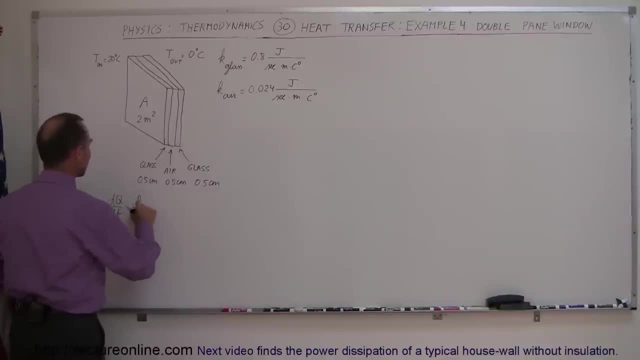 is equal to k, the heat conductivity constant times the cross-sectional area times the difference in the temperature between the outside inside, divided by the length of the path that the heat has to travel. But in this case, since there are more, since there's more than one layer, there's 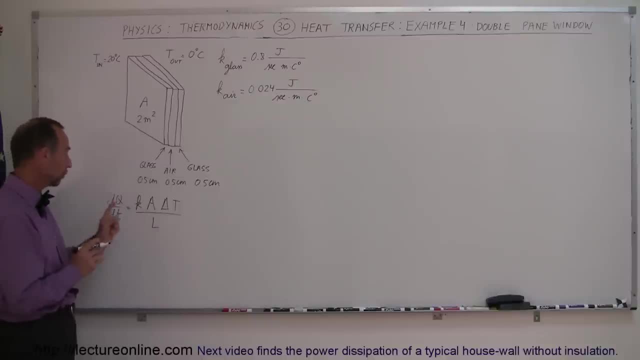 three layers. here we can use the equation as is. So what we're going to do here is take the k and break it down into the active heat. So we're going to take the heat and we're going to bring it down. So we're going to write this as A: the cross-sectional area times the. 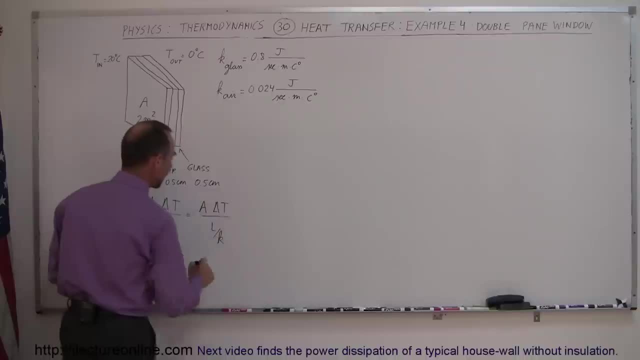 difference in the temperature divided by L divided by K. And since there are three layers, we need the L divided by K for all three layers. So really, what this becomes is this becomes equal to A times delta T divided by L1 over K1, plus L2 over K2, plus L3 over K3.. So, however, 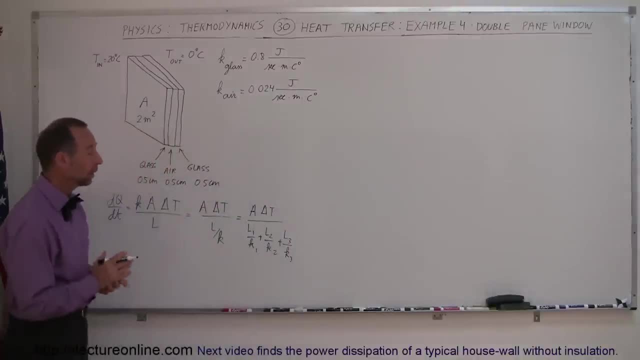 many layers there are, you need to have an L over K factor for each layer And, as we will see later on, that the L over K is a factor that is actually used in building materials and that's usually called the R rating, So the rating for the connectivity versus thickness. 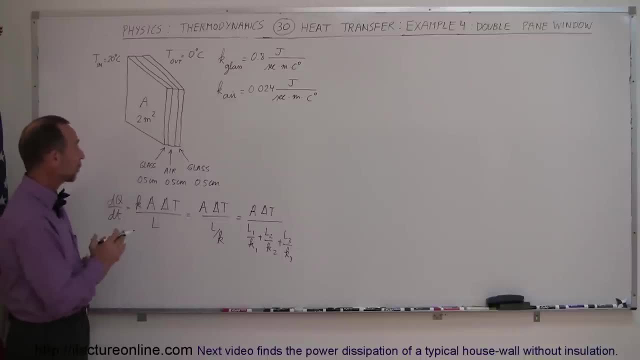 of the layer. All right, Now that we have the equation I want to use, let's plug in all the values. So this is equal to the, The area which is two meters squared times the difference in the temperature, which would be 20 centigrade degrees, divided by the L over K for each layer, Now the L1, notice. 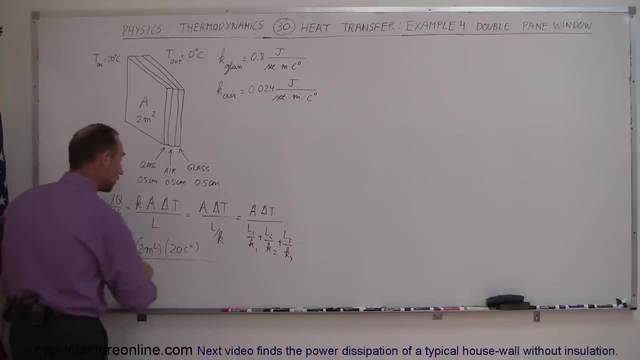 that each layer is a half a centimeter thick, So the L1 is 0.005 meters divided by the K1.. Now, since the first layer is glass, we use the 0.8.. So that's 0.8.. 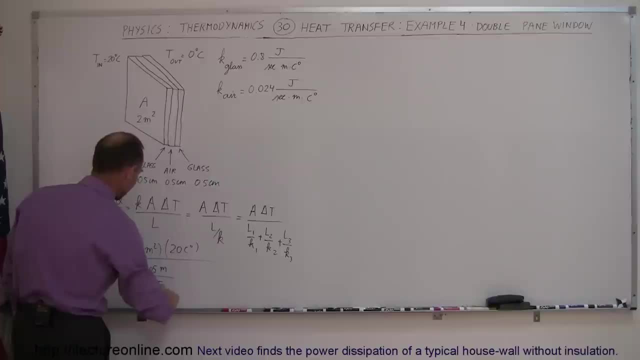 Joules per second, times meter times, centigrade degree, Okay, Plus. Now the next layer is air, And this is the beauty of a double pane window: The air is trapped between the two layers of glass And notice the heat conductivity for air is much smaller than the heat conductivity. 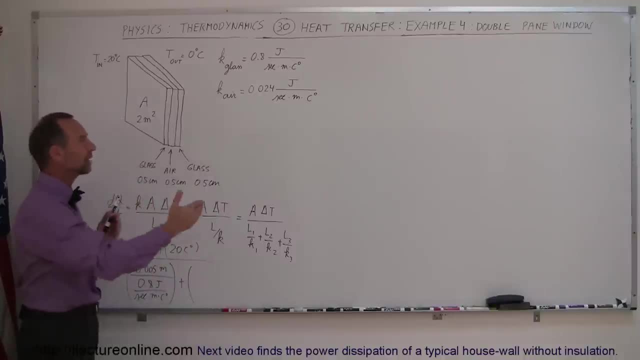 for glass, which is the insulating layer that makes it very difficult for heat to travel through a double pane window. So here we get 0.005 meters divided by 0.005 meters And we have 0.024 joules per second times meters, times centigrade degrees. Notice since this. 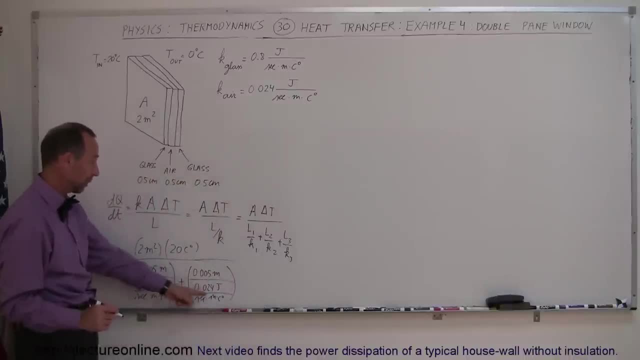 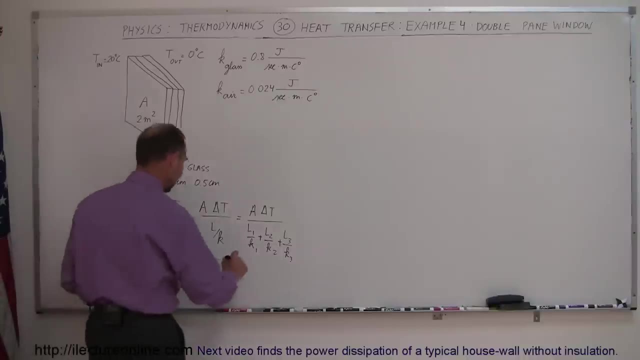 in itself will be a much bigger number, because 0.005 divided by this much smaller K will be a bigger number and therefore will make the overall fraction a smaller fraction. We still have our third layer, So we have plus, and that will be 0.005 meters divided by 0.8. 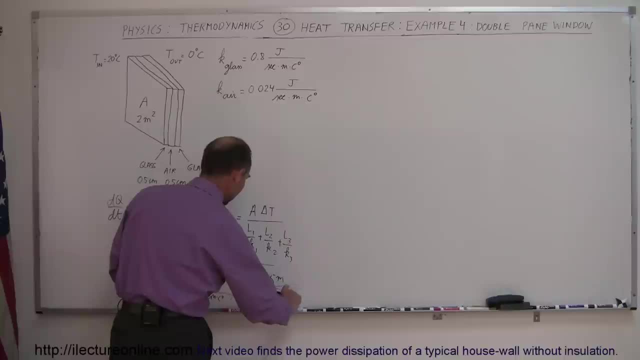 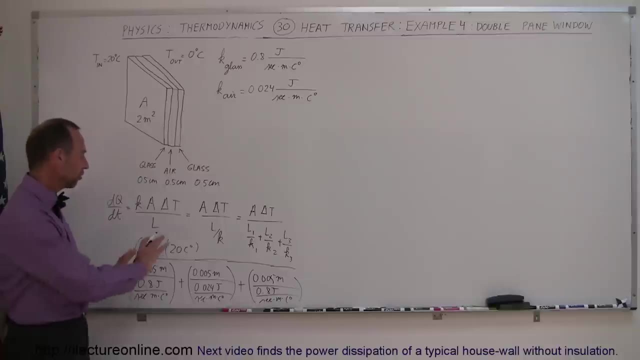 joules per second times meters. All right, It gets a little messy with all the units. Typically I would like to leave the units off, but just to make sure that when you simplify all the units you'll end up with joules per second or watts, So let's go ahead and calculate that. So in the denominator. 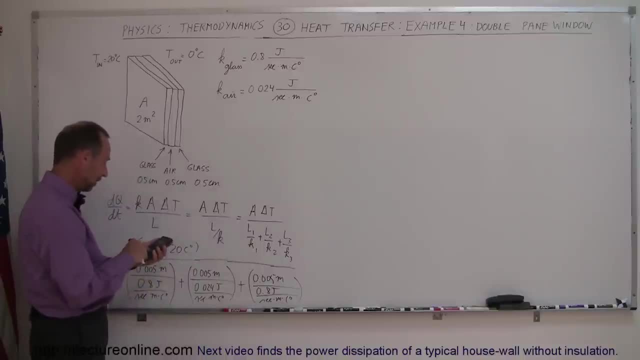 we have two of these terms. So we'll take 0.005 divided by 0.8 and double that, because there's two layers, And we add that to this following layer, which is 0.005 divided by 0.8 divided by 0.024 equals. so now that's the total sum of the denominator We push. 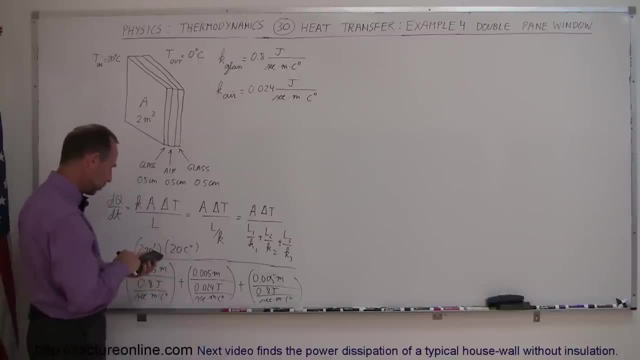 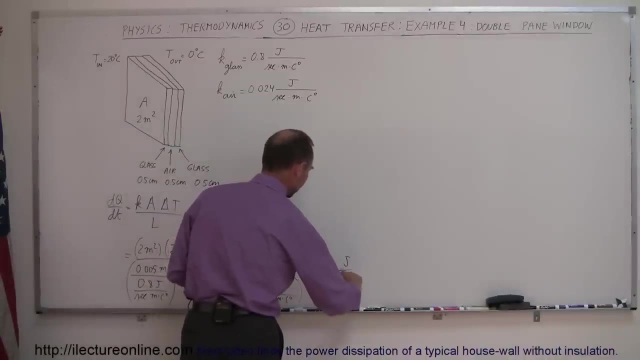 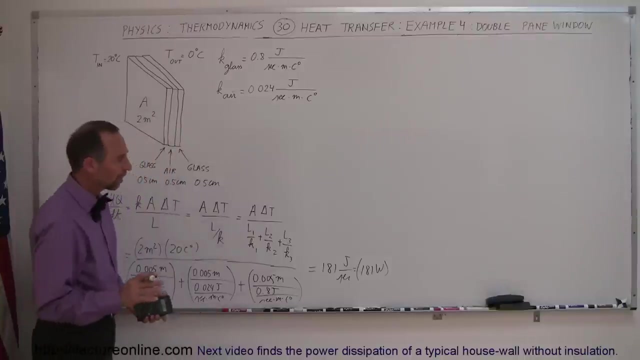 one over x on the calculator and then multiply that times two, and multiply that times 20, and we get 181 joules per second, which is equal to 181 watts. Now I don't know if you saw the previous video, but in the previous video we had a window. 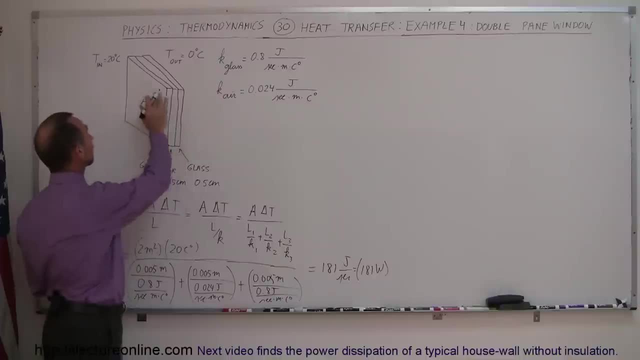 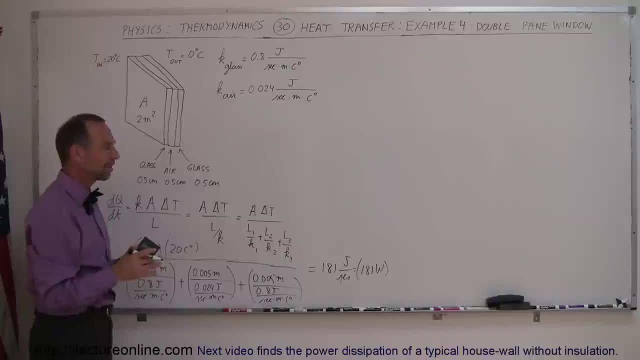 same cross-sectional area, same inside and outside temperature, And I believe the answer there was 6,400 watts. so notice the enormous reduction in heat loss through a double-pane window as compared to a single-pane window. So if you want to have a well-insulated house,